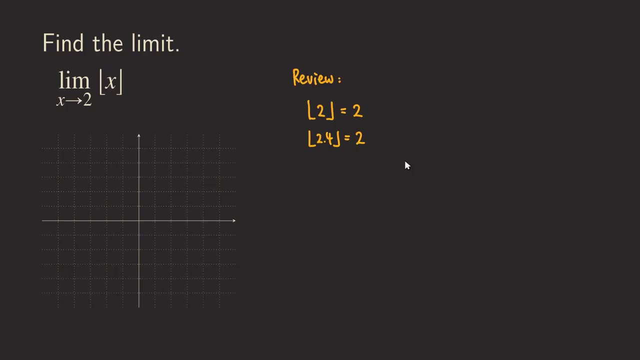 the largest integer that is less than 2.4 will just be 2, and then if we plug in, let's say, negative 4.6, for example, then what happens? we are going to also need to output in the largest integer that will be less than this number that we put into the function, so it would be negative 5.. Okay, so, 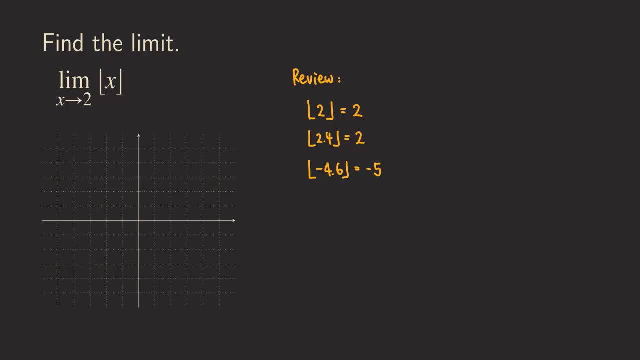 that's good. and then now we are going to grab the function, and so what happened is that we are going to, let's say, just imagine that we plug in things like 0.4, 0.1, 0.5.. Okay, so what happened is that. 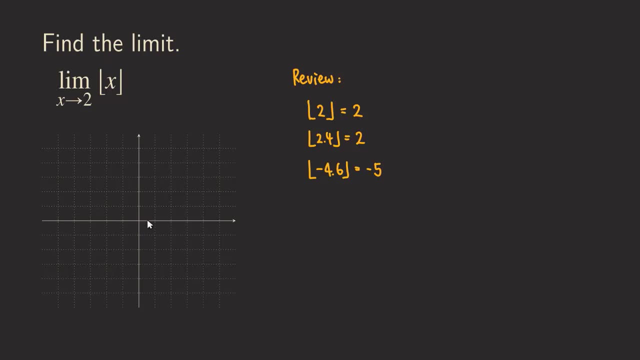 we. it will output the integer that is 0, because that 0 would be the last largest integer, less than all those numbers. so you see that we are going to, and then we put an open circle right here. it's that when we plug in a 1, we actually will get 1 right. so we are not going to get 0. so now we get this dot here and 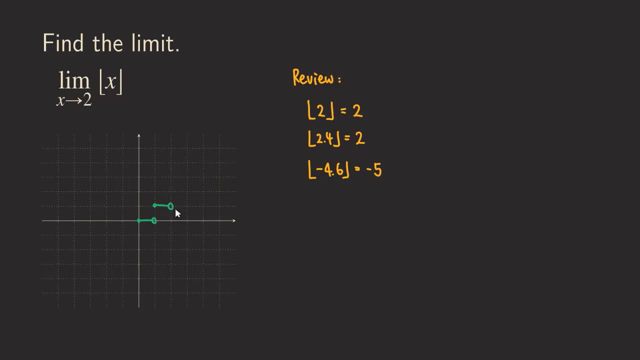 then just keep drawing it and then again open circle with this spot here, because when we get to 2 we are going to get 2. For the y value, so we are going to this one and then following the same pattern. then we can actually just grab all of them. 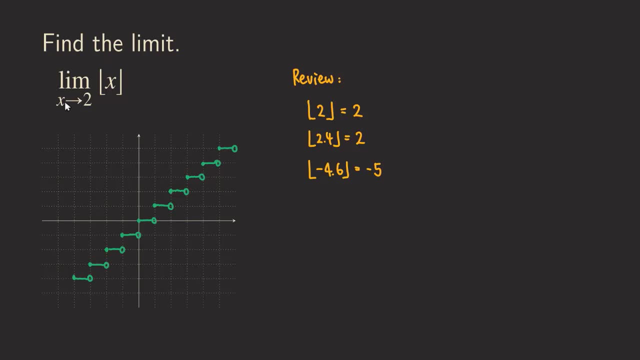 Well, actually we don't need that many pieces right here. it's really because we are just going to let x approach 2 right? so what we're looking at is actually this spot right here. so this is 2 right, so we are looking at this spot right here. so now what happened is that we are going to 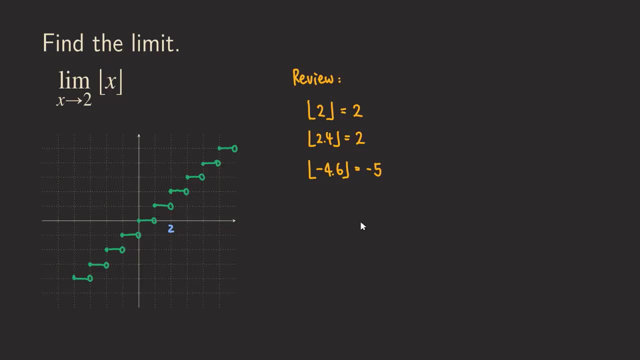 just compute the limit, let's say, if we are approaching 2 from the left side. okay, so let's just take the limit as x approaching 2 from the left side of this function. what happens is that we are going to get while based on a graph. then we are going to just get what if you draw some arrows. 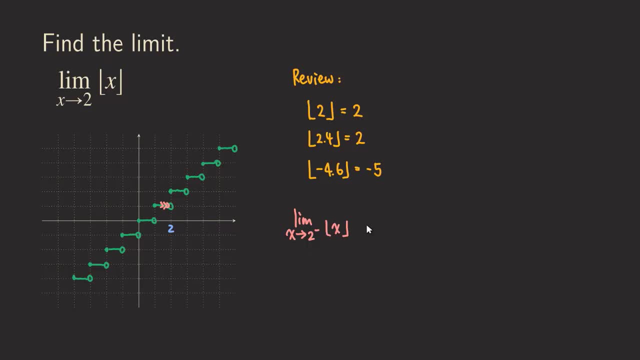 right here. you can see that it's approaching 1. okay, so we just get 1 right here. and then, on the other hand, if you are approaching 2 from the right side, then let's just draw some arrows right here. what happens then? the function will be approaching what 2? so we get 2 here, and then you can see that those two one-sided.